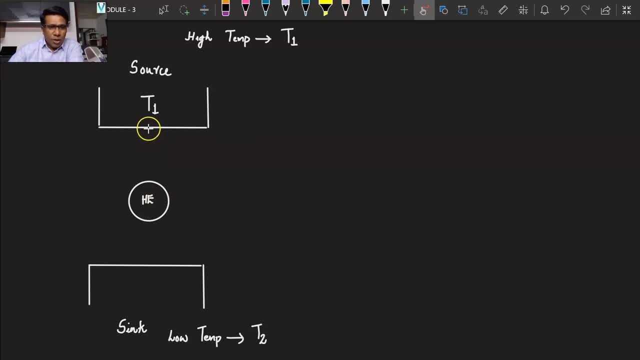 Now, how does it work? The heat engine absorbs heat from the source. Okay, it is absorbing the heat, So I am marking it as Q1.. Q1 is the amount of heat that is being absorbed. It absorbs and converts a portion of this heat to work, to positive work. 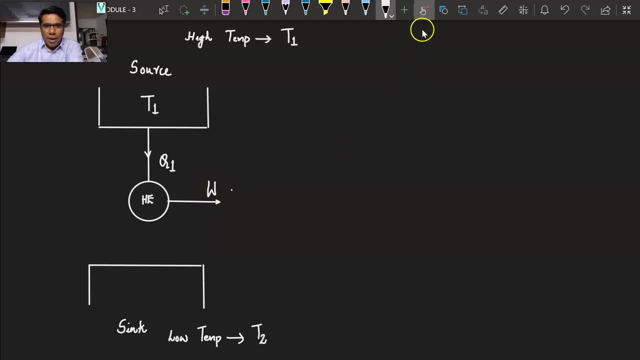 So I am denoting it by W and the remaining will be rejected to the sink. that is the atmosphere, Say. I am representing it by Q2.. So this block diagram is now completed. The heat engine it absorbs. 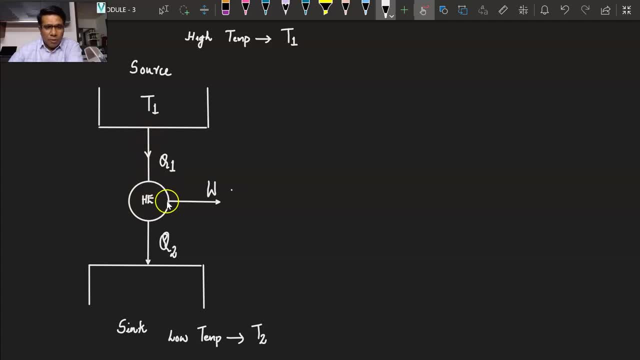 It absorbs heat from the high temperature source, convert a portion of it into work and the remaining heat is rejected to the sink, which is kept at the temperature T2.. That is the basic functioning of a heat engine. Now the efficiency of a heat engine. 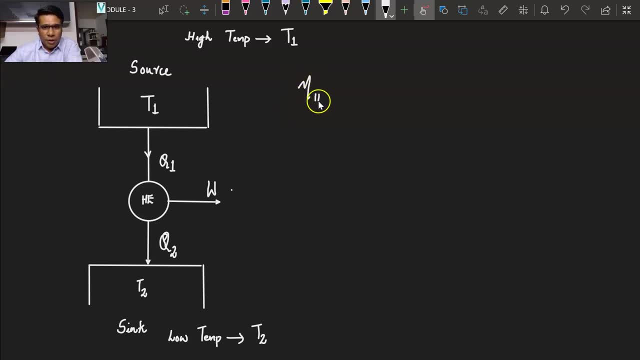 I am going to do the efficiency of the heat engine. Efficiency is always represented by the desired temperature. That is the desired output By the required input. This is a standard efficiency statement: Desired output by the required input. Now, if you look at the heat engine, the desired output. 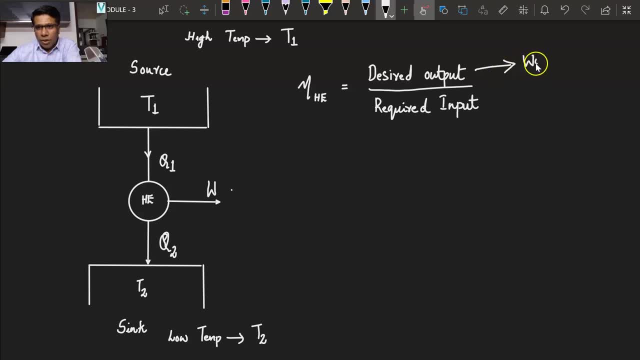 What is the desired output? The desired output of the engine is work And what is the required input? I need to input Heat. is the input, The input heat, not the rejected heat. The input heat is the required input. Therefore, I can see that I have represented Q1 as the heat which is absorbed. 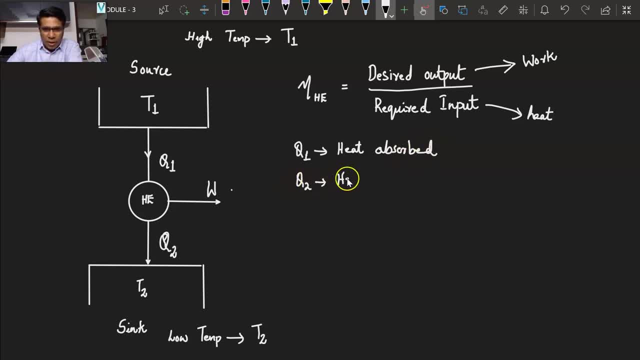 And Q2 is the heat that is rejected. Therefore, efficiency of a heat engine is the required input. Therefore, efficiency of a heat engine is equal to what is the desired output. It is the work divided by the desired input is the heat absorbed. 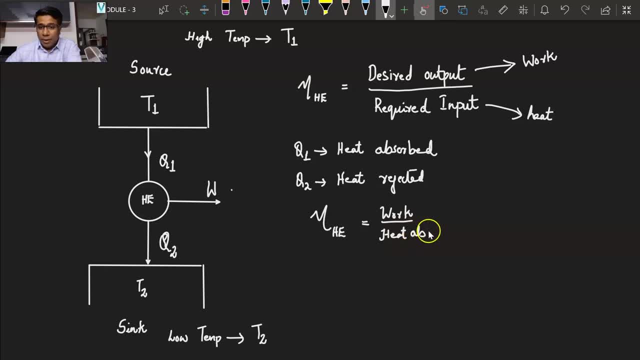 There is no heat rejected in the required input condition. Therefore it is heat absorbed. So it becomes W by Q1.. And in case of a reversed heat engine, We are considering the theoretical case where the work done is equal to the Q1 minus Q2.. 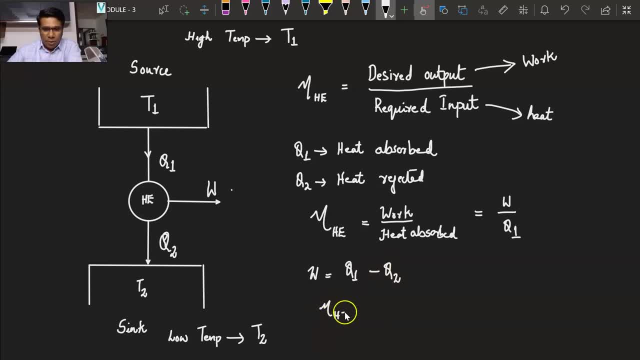 So the efficiency equation can be written as W, that is, Q1 minus Q2 by Q1.. Or it can be written as 1 minus Q2.. Now, this is the fundamental equation that we can use for a heat engine, when we know the heat absorbed and the heat rejected. 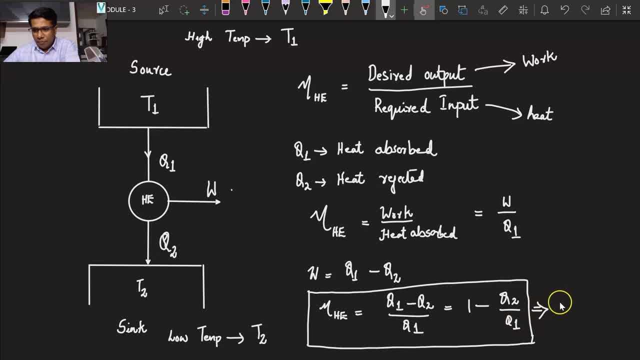 Now this can be written as 1 minus T2 by T1 in case of a reversible cycle or in case of a reversible heat engine, And this will be proved by the thermodynamic temperature scale. But this is also, again, a very possible equation that can be used for any reversible heat engine. 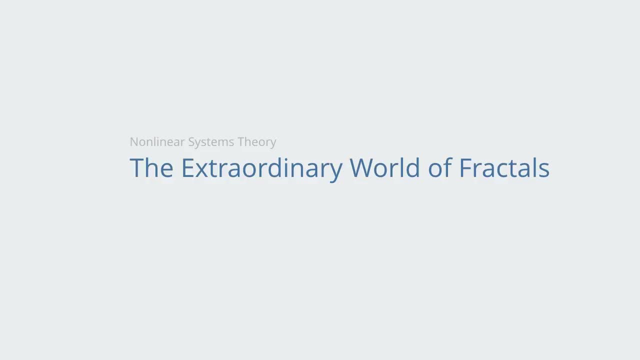 Fractals are sometimes called the pictures of nature, and if chaos theory, as the name implies, is the chaotic and unpredictable dimension to non-linear systems, then we might say fractals represent their orderly side. We see lots of order in our world, The earth. 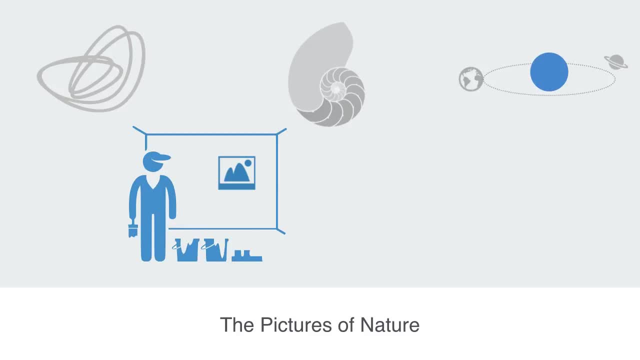 goes round the sun today and it will do the same tomorrow and the next day for millions of years. If we take a butterfly, we see that one side of it is almost exactly mirrored in the other. We see the same in the regular geometric forms of snowflakes, One way of 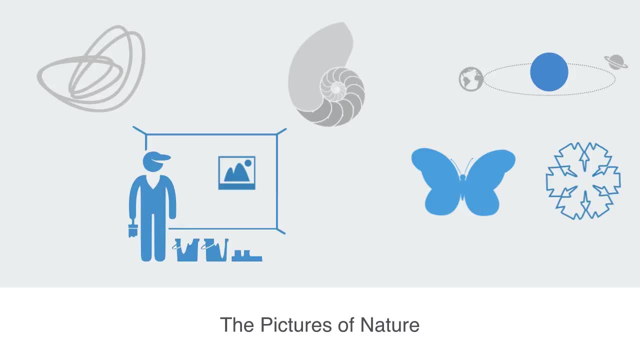 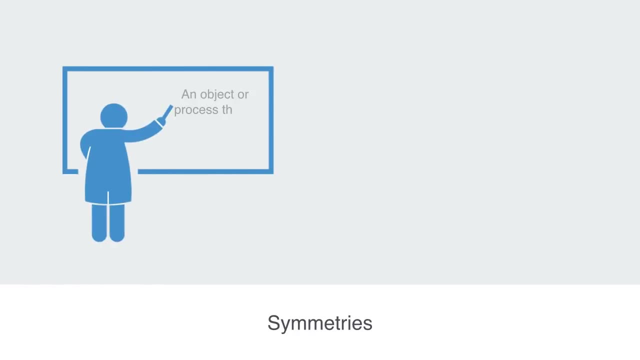 understanding this order is through the concept of symmetry. In mathematics, symmetry can be defined as an object or process that is invariant to a transformation. In more familiar terms, this means something that stays the same despite a change. So with our example of the butterfly, its external,